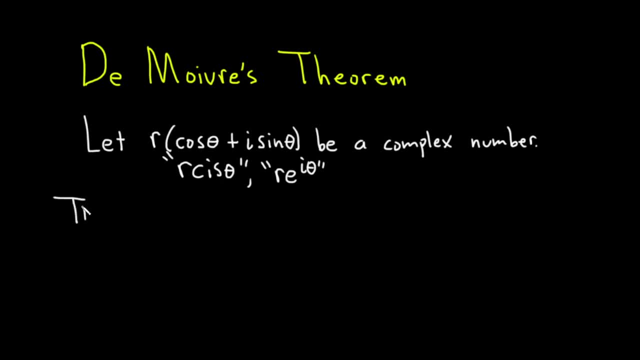 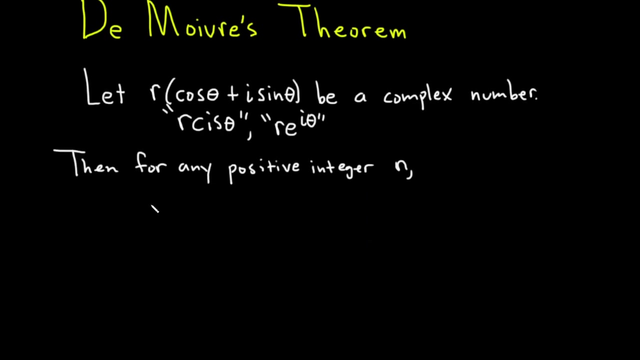 that follows Then for any positive integer n. so for any positive integer n, we have the following: We can raise this complex number to a power in a very convenient way. So I'm going to use a different color here and I'm going to write down all three. 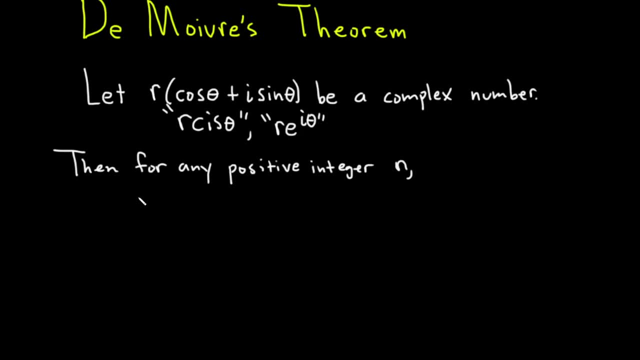 varieties. so you can see how all of these are applied. For the first one, we'll use a bracket here: Bracket r, cosine theta plus i sine theta- parenthesis- and then bracket. So if you raised this to the nth place, that will be the shape lookin' like this: The nth. 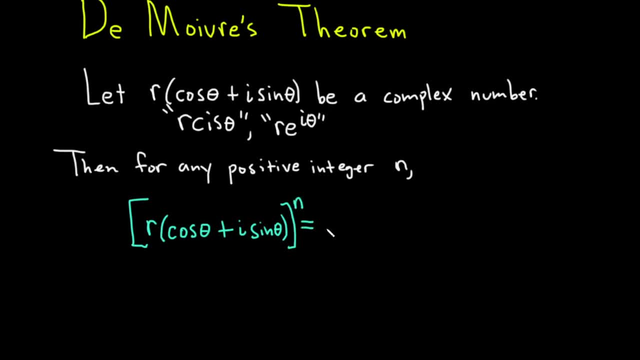 this to the nth power. you basically raise the r to the nth power and then the n goes inside. the trig functions like this Cosine of n? theta. It's pretty cool. Plus i sine n theta. Really really cool theorem, I think So. 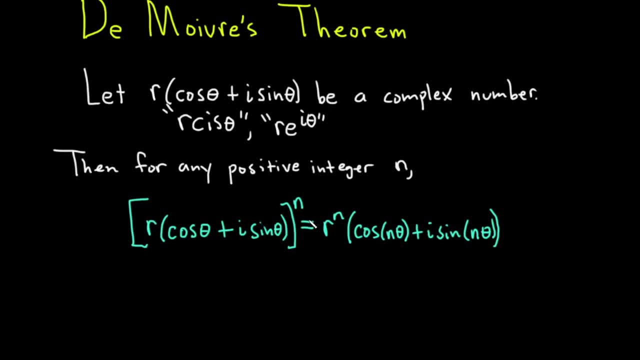 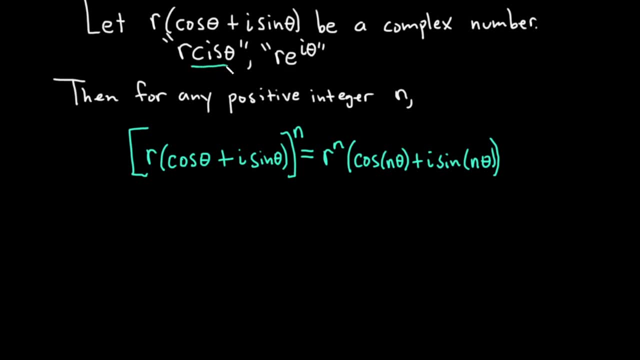 really powerful And we'll do an example in a minute. It's actually really simple to use. Alternatively, if we use the SIS notation- by the way, SIS stands for cosine i sine- This would be bracket R, SIS theta. I guess I don't need the 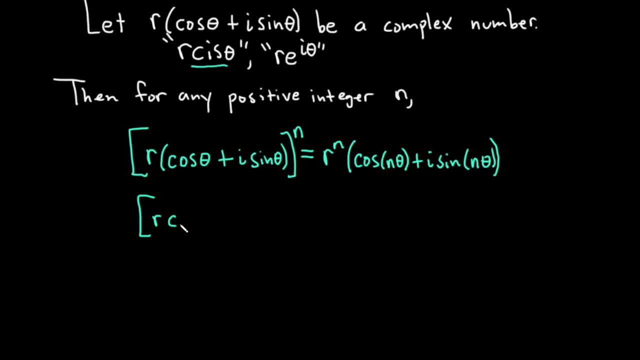 parentheses there. Let me get rid of that, since it's just SIS. It makes it a little bit cleaner. SIS theta. And again we're raising this to the nth power. You get r to the n SIS n theta. Okay, And just to be. 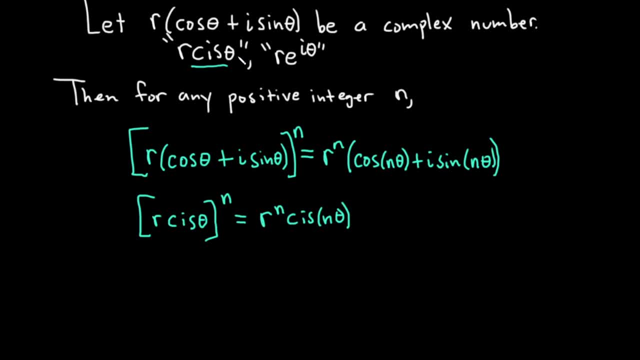 really clear to make sure there's no confusion. what is SIS theta, So SIS theta. maybe I'll write it up here: SIS theta is cosine i sine, So it's cosine theta plus i sine theta, So it's exactly the same thing as what you see here. So this is SIS Likewise. 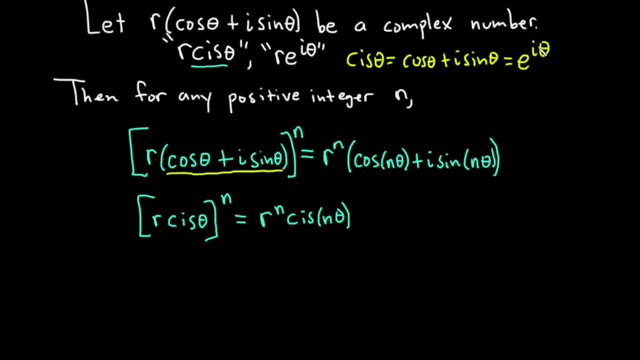 this is also equal to e to the i theta. So same thing. All of these are exactly the same Here with De Moor's, let's write it down using this exponential notation: So we have r? e to the i theta And that's being raised to the nth power, And this would be r to the. 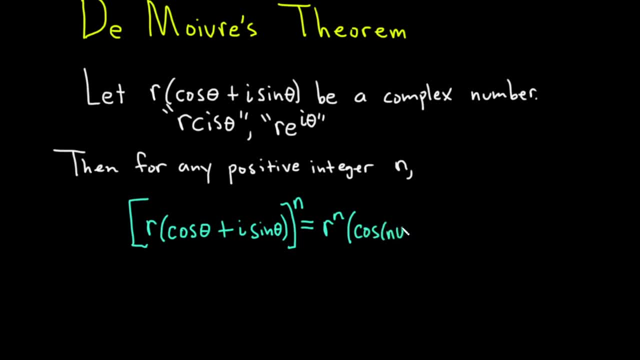 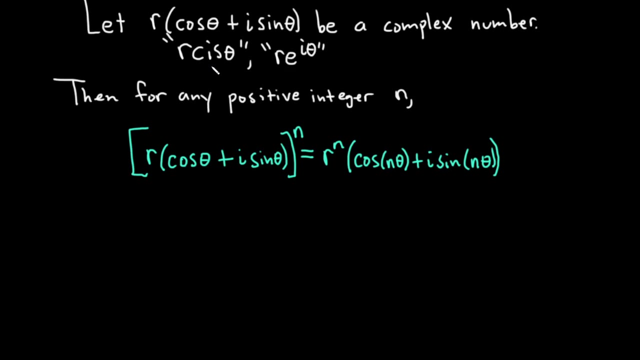 like this Cosine of n? theta. It's pretty cool. Plus i sine n theta- Really really cool theorem, I think, So really powerful, And we'll do an example in a minute. It's actually really simple to use. Alternatively, if we use the cis notation- by the way, cis stands for cosine i sine. 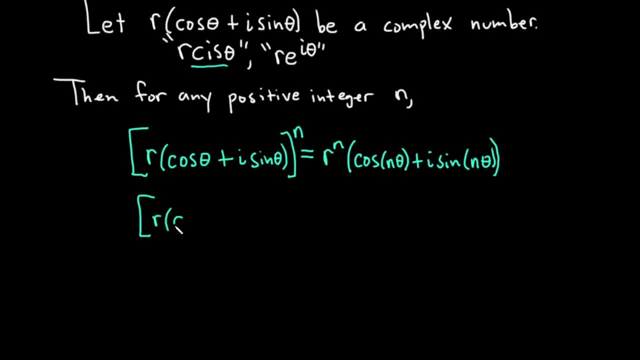 This would be bracket r. cis theta. I guess I don't need the parentheses there. Let me get rid of that, since it's just cis. It makes it a little bit cleaner- Cis theta. And again we're raising this to the nth power. You get r to the n. 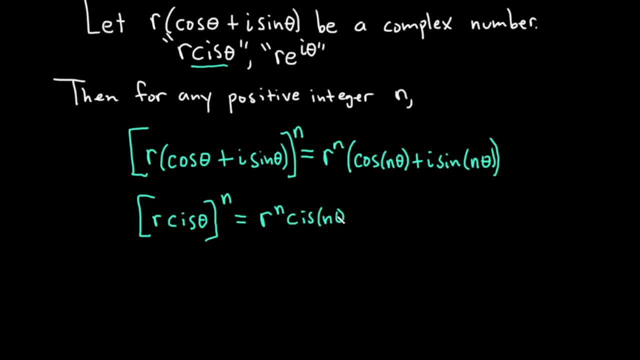 Cis n theta. Okay, And just to be really clear, to make sure there's no confusion: what is cis theta, So cis theta? maybe I'll write it up here: Cis theta is cosine, i sine, So it's cosine theta plus i sine theta, So it's exactly the same thing. 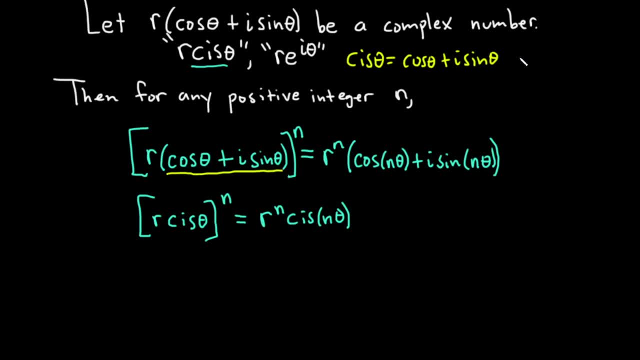 as what you see here. So this is cis. Likewise, this is also equal to e to the i? theta. So same thing, right, Same thing. All of these are exactly the same. So, continuing here with De Moor's, let's write it down using this exponential notation: So we have r? e to the i. 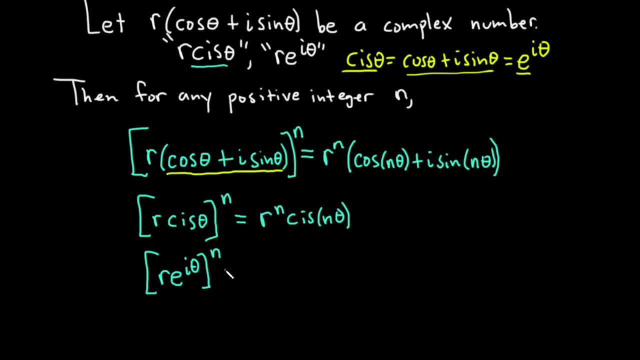 theta And that's being raised to the nth power And this would be r to the n, e to the i n theta. This makes more sense for a lot of people. You're basically exponentiating the e right n times i theta is, you know, n times i theta. So you're basically exponentiating the e right n times i. 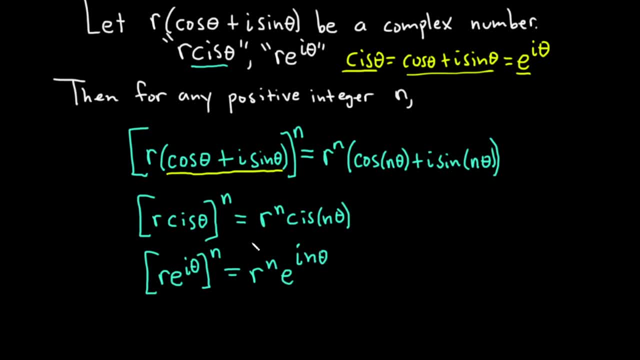 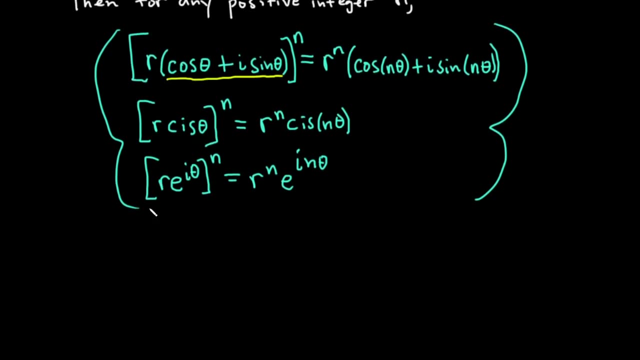 theta, which is right here n times i theta. So algebraically, this is the one that makes the most sense for people. So all of these, all three of these, are considered De Moor's theorem. So let's go ahead and just do a simple example of using De Moor's theorem to raise a complex number. 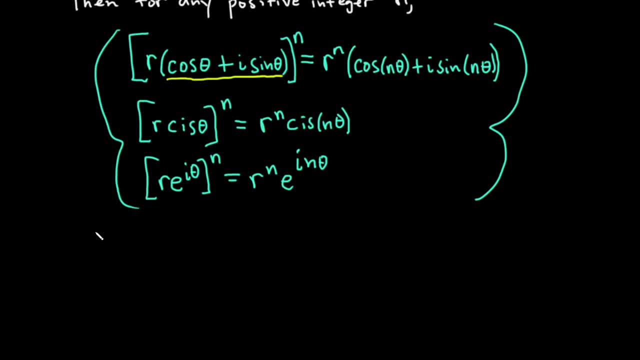 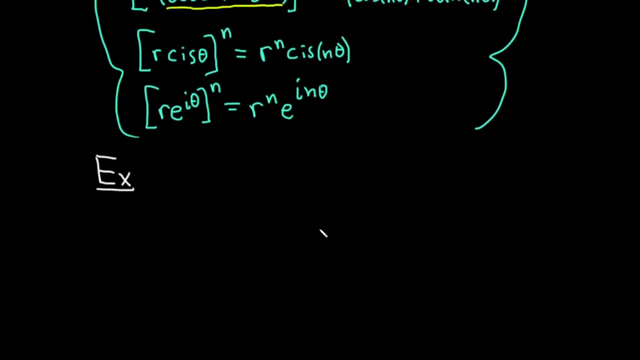 to a power And typically when you do these, like in a classroom setting, they always say: don't use a calculator. you know, do it by hand, show all your work. But it's pretty, it's pretty simple. So let's start maybe with this. one: say: we have bracket three parentheses, cosine And. 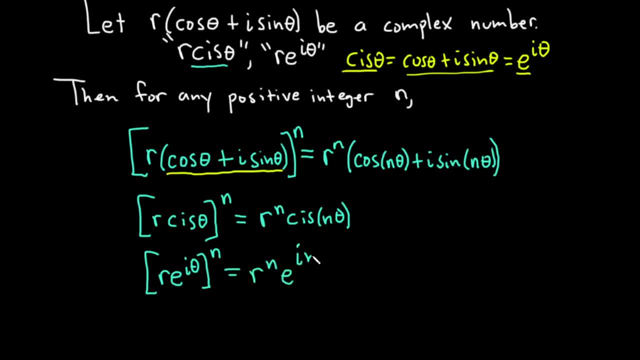 n e to the i n theta, And this makes more sense for a lot of people. You're basically exponentiating the e right n times i theta is you know, n times i theta, which is right here n times i theta. So algebraically, this is the one that makes the most sense for people. 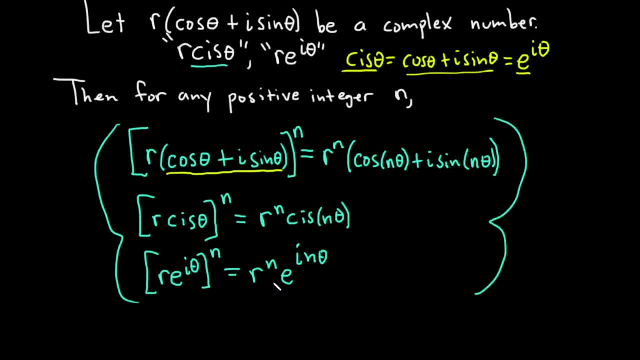 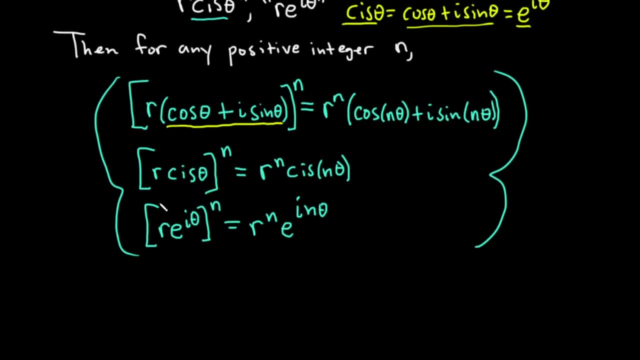 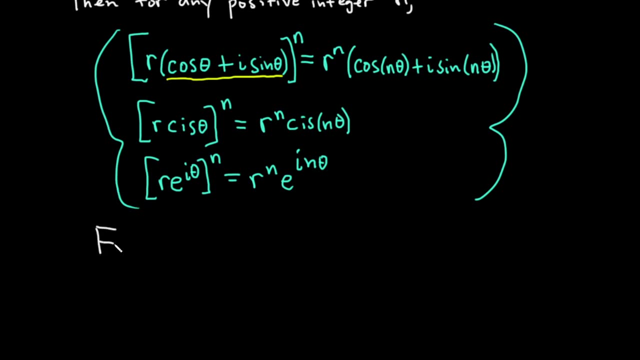 So all of these, all three of these are considered De Moor's theorem. So let's go ahead and just do a simple example of using De Moor's theorem to raise a complex number to a power. And typically when you do these, like in a classroom setting, they always say: 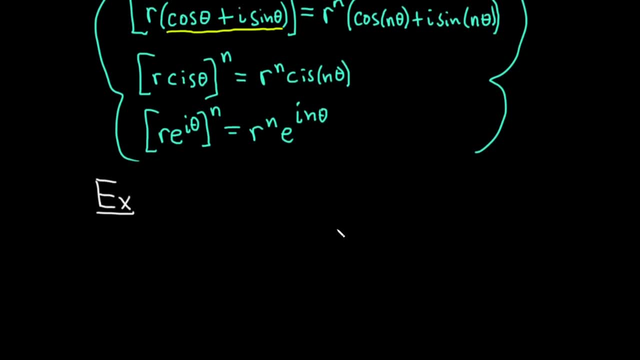 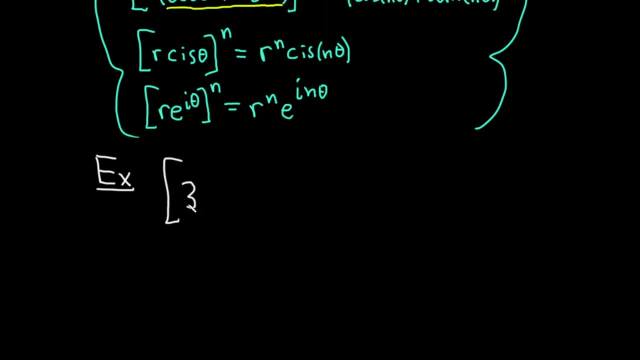 don't use a calculator, you know, do it by hand, show all your work. But it's pretty, it's pretty simple. So let's start maybe with this one: say we have bracket, three Parentheses, cosine, And let's do three pi over four, So three pi over four. 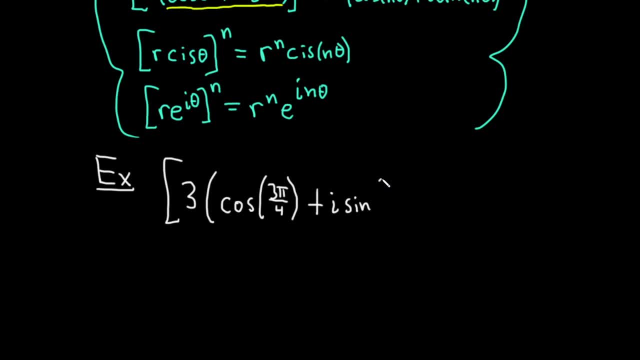 Plus, i sine three pi over four Parentheses and then I guess we need one more parentheses here. All right, to match this one here and then, and then a bracket, and we're going to raise this to the fourth power. We're going to go to the fourth power this time. All right, let's go ahead and go through it. 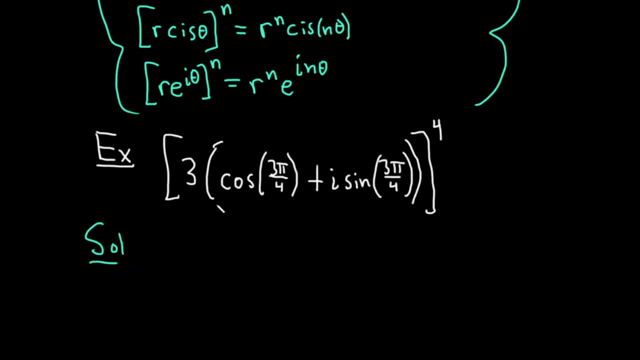 So solution: pretty easy. All we do is using the formula. we raise the R right. this is our oops, this is our R. So that will be three to the fourth, And then the four goes inside the trig functions, So it'll be cosine of four times three. pi over four, that's your n plus i. 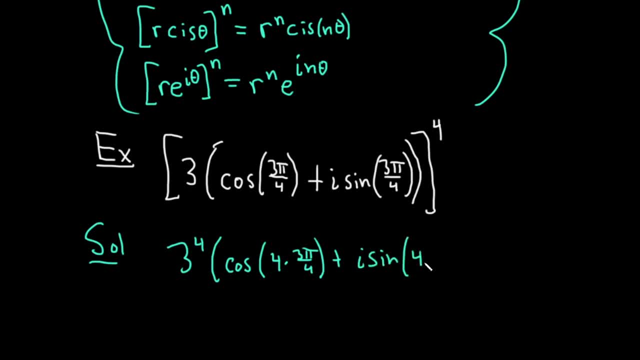 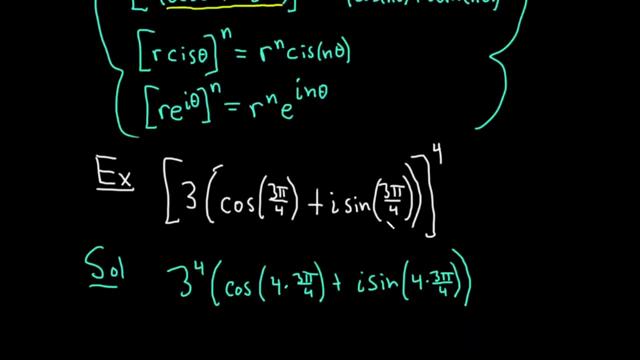 sine of four. Okay, just like that, And let me just show you the formula up here, just so you can see we're using it correctly. So it's R to the n, and then cosine n theta, i sine n? theta. So it's three to the n, n is 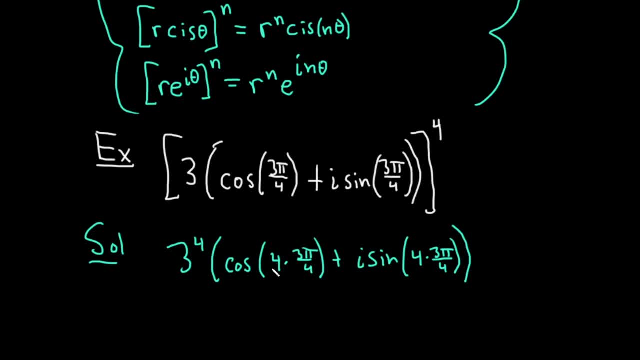 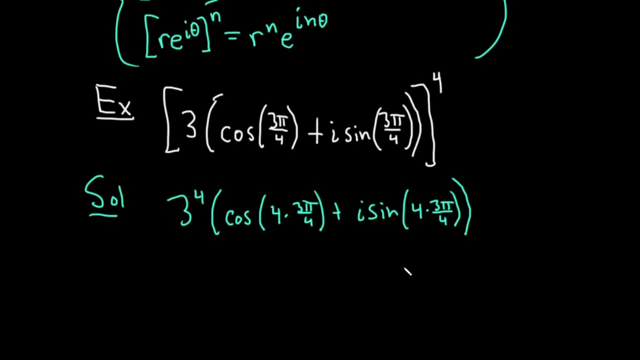 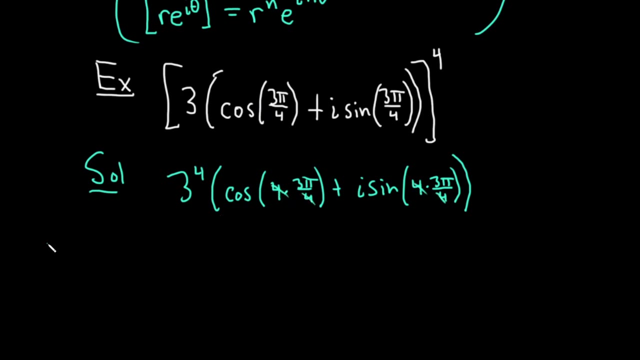 four here. cosine n theta, So n is four. theta is three pi over four. i sine n theta n is four. theta is three pi over four. So very simple. So now we can clean this up, we can cancel these fours. Three to the fourth is 81.. That's because it's three squared times three. 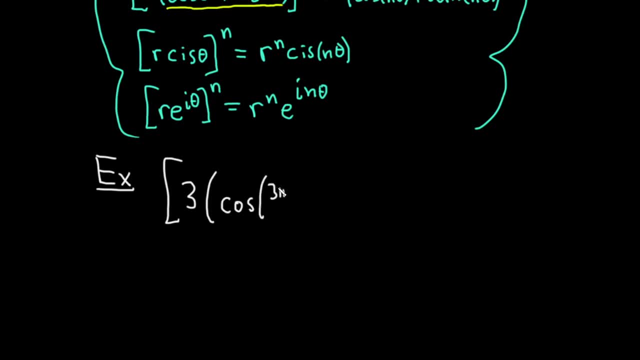 let's do three pi over four, three pi over four plus i sine three pi over four parentheses, and then I guess we need one more parentheses here Right to match this one here And then, and then a bracket, And we're going to raise this to the. 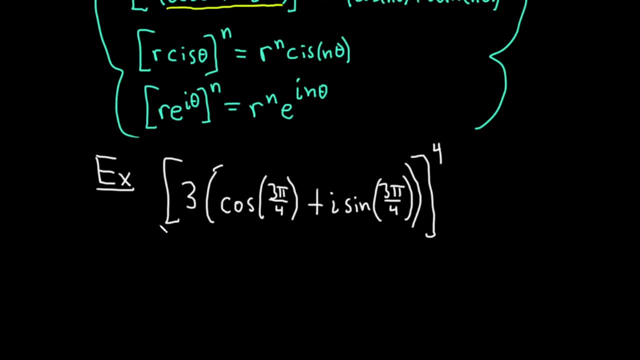 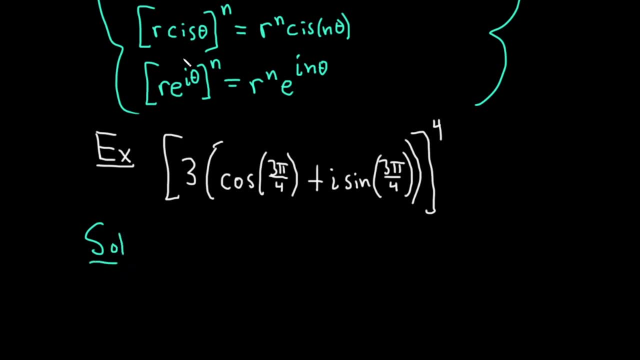 fourth power And we're going to go to the fourth power this time. All right, let's go ahead and go through it. So solution: pretty easy. All we do is using the formula: we raise the R right. this is: 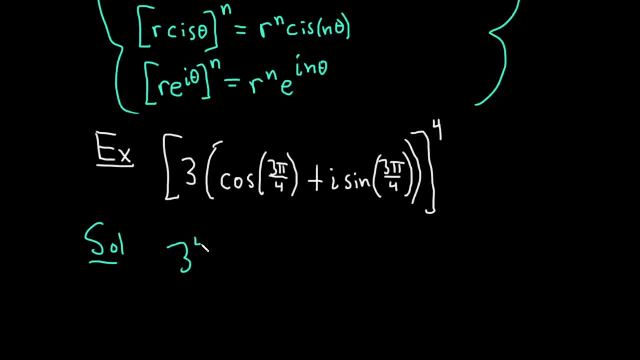 our oops, this is our R, So that will be three to the fourth, And then the four goes inside the trig functions, So it'll be cosine of four times three pi over four. That's your n plus i, sine of four times three pi over four. Okay, just like that. And let me just 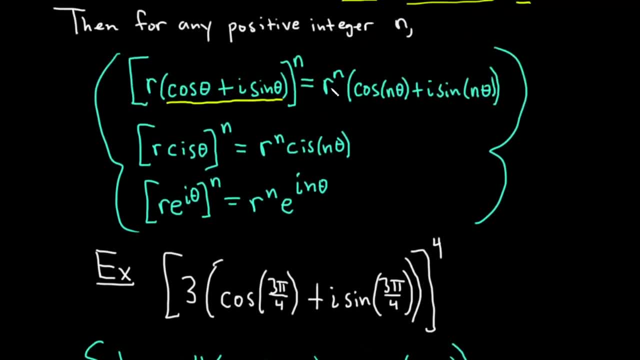 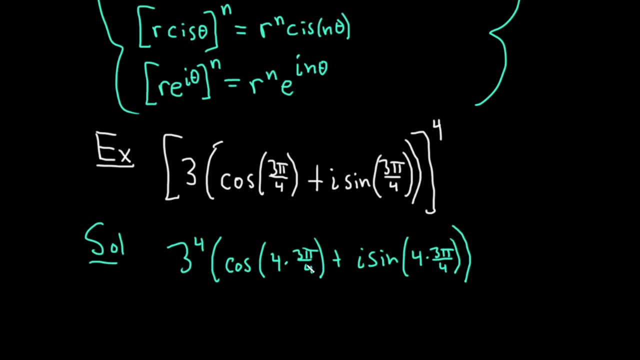 show you the formula up here, just so you can see we're using it correctly. So it's r to the n, and then cosine n theta, i sine n theta. So it's three to the n. n is four here. cosine n theta So. 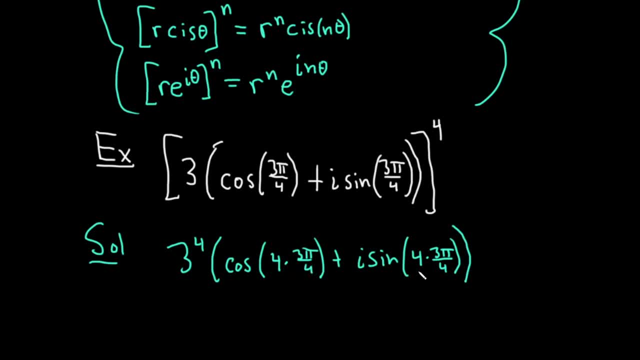 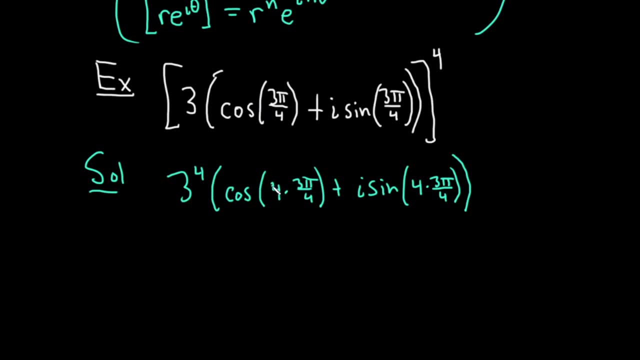 n is four, theta three pi over four. i sine n. theta n is four, theta is three pi over four. So very simple. So now we can clean this up, we can cancel these fours. Three to the fourth is 81.. That's because it's three squared times. 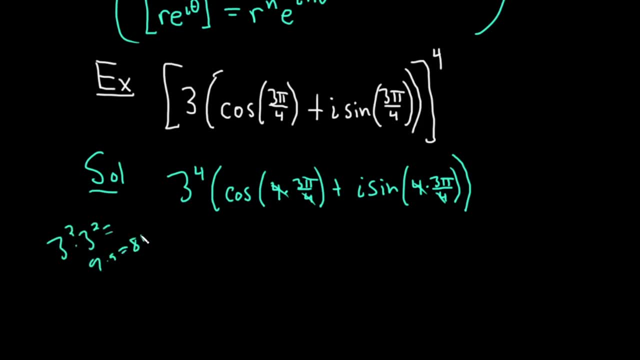 three squared, which is nine times nine, which is 81.. So pretty simple. So it's 81.. Then we get the cosine of three pi, plus i sine three pi. So to figure out the cosine of three pi, we're going to use the formula, we're going to use the 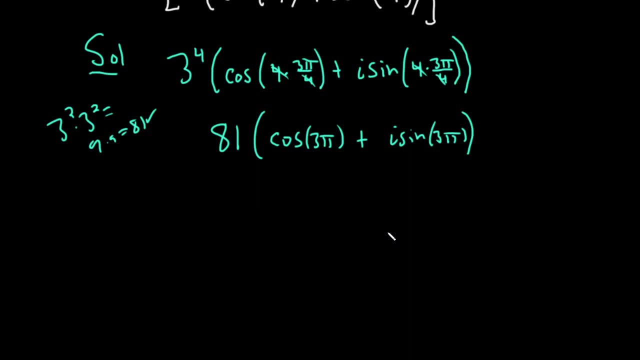 formula to figure out what the cosine of three pi is and what the sine of three pi is. what we can do is think about the unit circle. So I'll draw a picture here Here's. here's the unit circle. the unit circle is a circle of radius, one centered at the origin, And the unit circle is special. 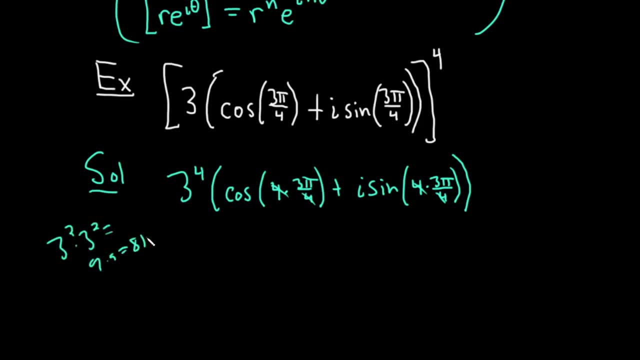 squared, which is nine times nine, which is 81.. So pretty simple. So it's 81.. Then we get the cosine of three pi, plus i sine three pi. So to figure out what the cosine of three pi is and what the 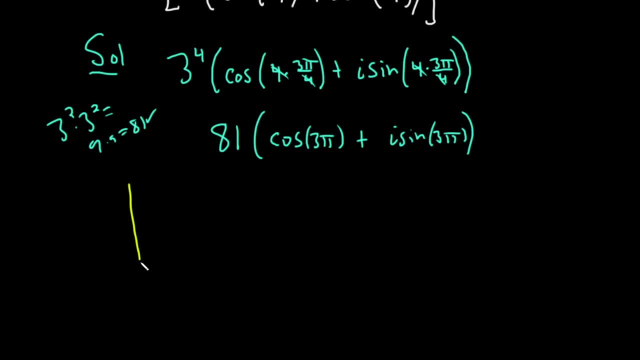 sine of three pi is what we can do is take the cosine of three pi, and what we can do is take the cosine of three pi, and what we can do is even add the sine. So first we're going to query the unit circle. So here's the unit circles. so I'll draw a picture here. So here's, here's the unit. 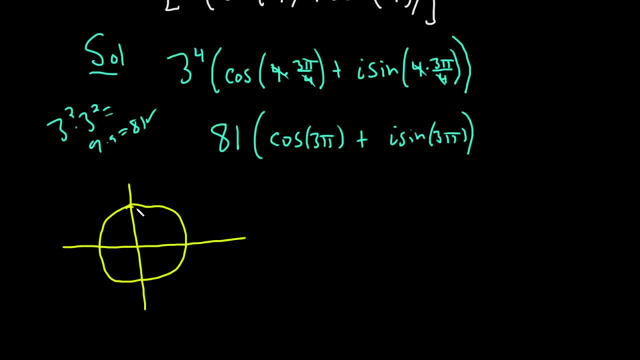 circle. The unit circle, is a circle of radius, one centered at the origin. And the unit circle is special because every ordered pair on the unit circle has the form cosine, theta, comma sine theta. So here this is zero, but it's also two pi. So to get to three pi you do one complete. 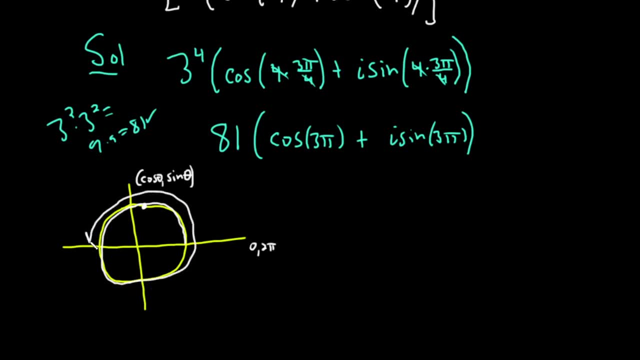 revolution go one more half revolution. So this would be 3 pi, which is also pi. So we want the ordered pair here. Well, because it's the unit circle, this distance here is 1.. So the x-coordinate is negative 1.. And you can see, here we're on the x-axis, So we're going up by 0.. So the y-coordinate 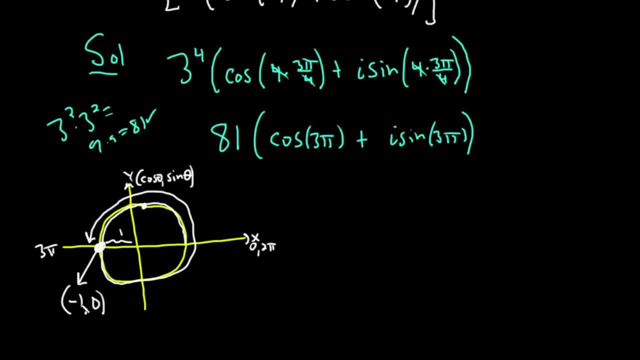 is 1.. Cosine is the x-coordinate on the unit circle. So cosine of 3 pi would be negative 1, because that's the x-coordinate. This is 81 times negative 1 plus i times And then sine of 3 pi. 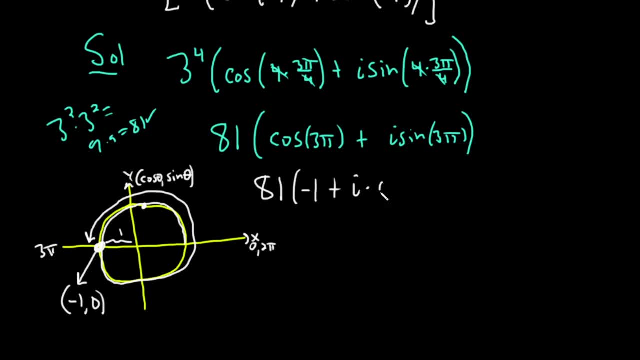 would be the y-coordinate at 3 pi, which is 0. So this is just 0. So we get 81 times negative 1 plus 0. And so we get the answer of negative 81, which is really really nice. So that's how you. 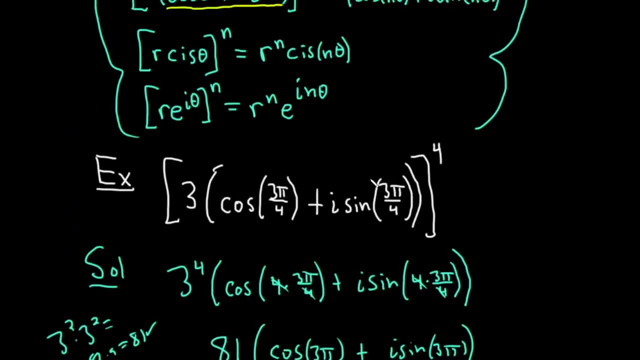 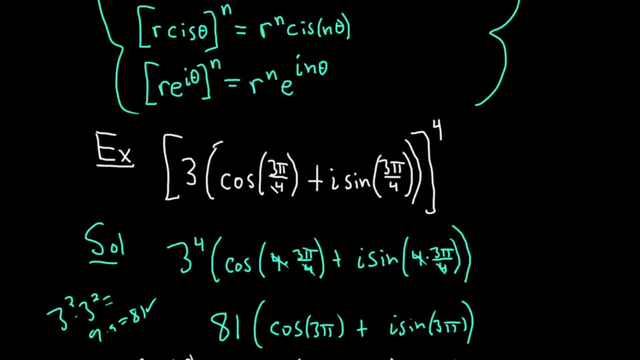 use DeMoore's theorem. And yeah, it's pretty simple. All you do again is you just raise r- This is your r- to this power, And then you just put the number inside the trig functions, And then you clean it up, And after that you're good to go. 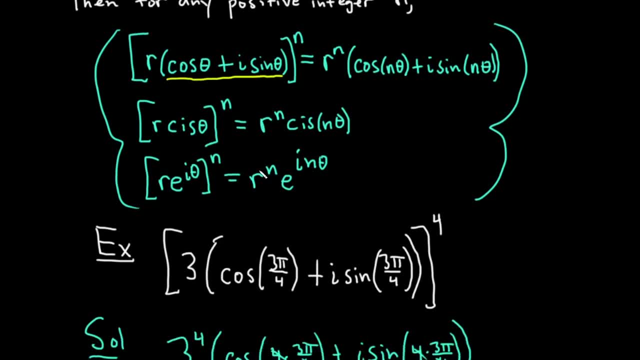 Remember r is called the modulus And theta is called the argument of the complex number. I hope this video has been helpful. Good luck.